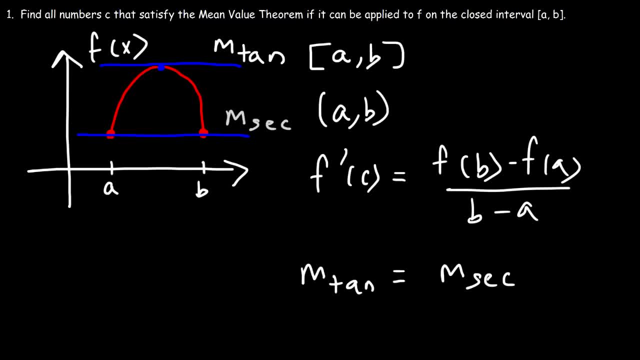 The tangent line only touches the curve at one point. So therefore C is right in the middle between A and B in this example. So anytime you have a closed interval, if the function is continuous on a closed interval and if it's differentiable on the open interval. 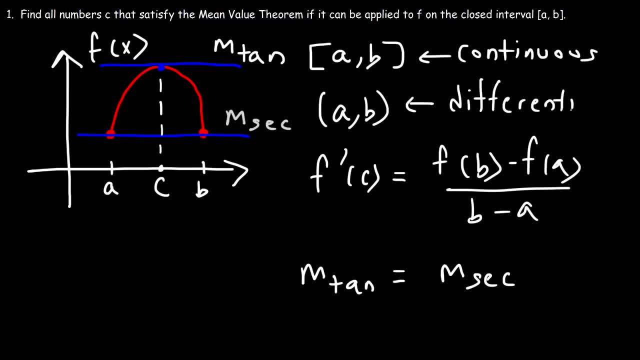 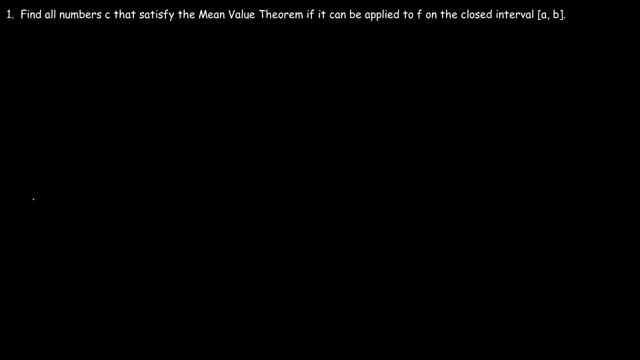 there's always going to be some number C where the slope of the tangent line is equal to the slope of the secant line, where those two lines will be parallel to each other. Now let's look at another graphical example. So let's say: this time we have a graph that looks like this: 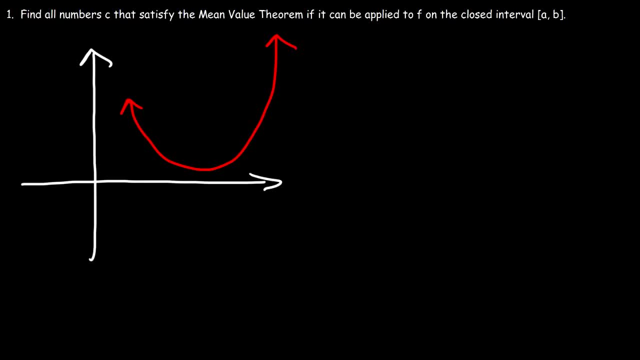 And let's say: here's A and here's B. Now is the function continuous on the closed interval? Yes, it is. There's no jumps, no discontinuities, no vertical asymptotes. Is it differentiable on the open interval? 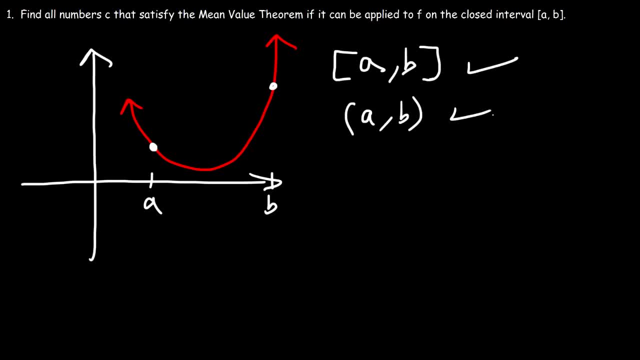 Yes, it is. There are no sharp turns in this graph. So therefore we could say that the instantaneous rate of change at C will equal the average rate of change between A and B. So in other words, the tangent line is going to be parallel to the secant line. 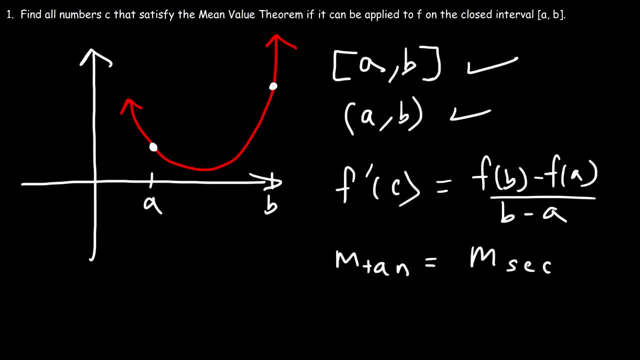 So the slopes of the tangent line and the secant line will be equal to each other. Now you've seen this equation. in this form, The slope between two points is y2 minus y1 divided by x2 minus x1.. And f is always equal to y. 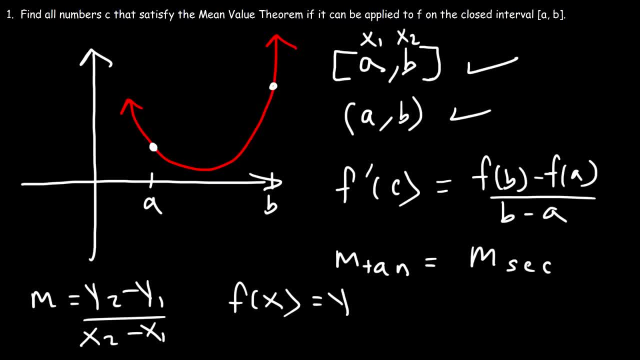 So this is x1 and x2.. A and B are x values, Whereas f of B, that's going to be y2.. And f of A is y1. So this is basically the slope between two points. That's where it comes from. 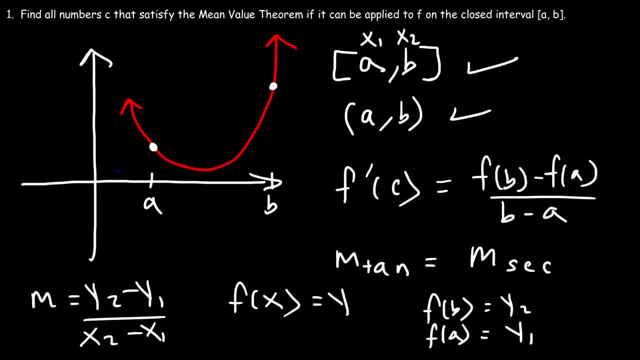 Now let's draw the secant line. So the secant line, as you mentioned before, touches two points on the curve. Now what do you think? point C is such that it's going to be parallel to the secant line. 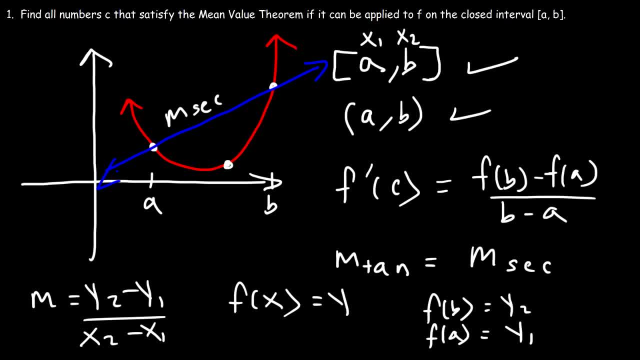 C has to be somewhere in this region, Because if we draw the tangent line, it can only touch the curve at one point. So notice that these two lines are parallel to each other. So that's what the Mean Value Theorem helps us to do. 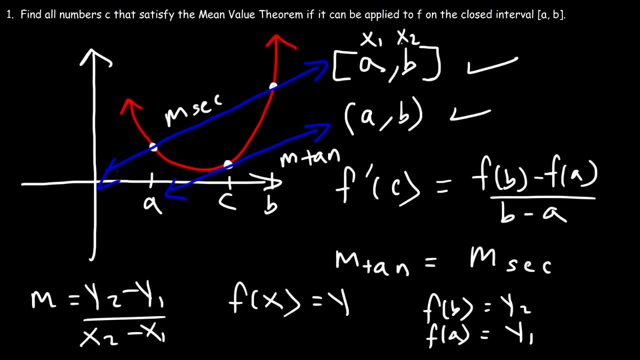 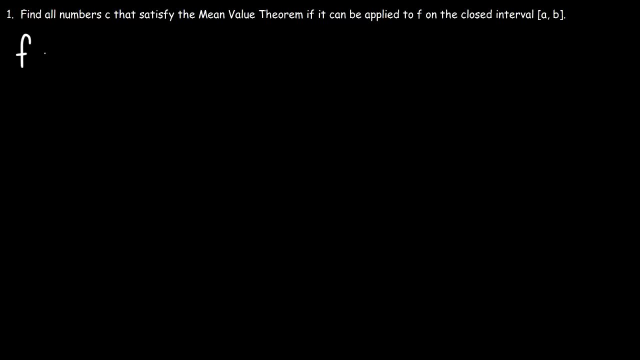 It helps us to find some value C between A and B where the slope of the tangent line is equal to the slope of the secant line. So now let's work on some problems. So let's say that f of x is equal to x squared minus 4x plus 1 on the interval 1 to 5.. 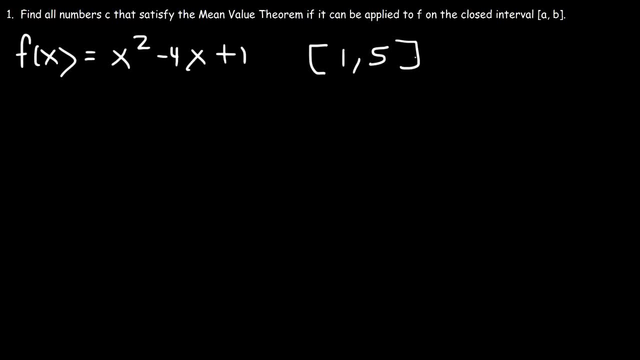 So first Can we apply the Mean Value Theorem to this function on its interval. Now the parent function, x squared, looks like this: It's basically a parabola. Now it's been shifted to the right, And so we can still see that for any parabola it's always going to be continuous everywhere and differentiable everywhere. 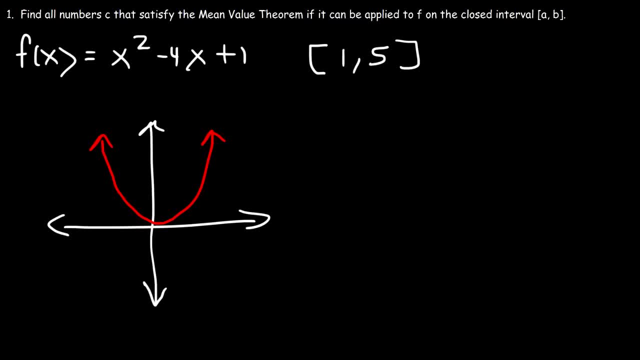 There's no sharp turns And there's no discontinuities. So for any type of polynomial function, be it a cubic function, a quadratic function, a linear function, they're all continuous and differentiable. So the Mean Value Theorem can be applied to those functions. 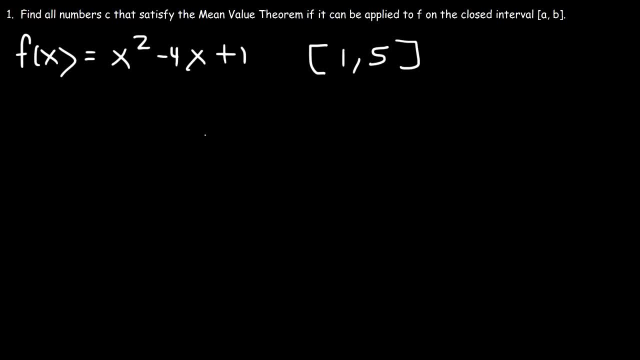 So all we need to do now is apply this formula: f prime of c is equal to f of b minus f of a over b minus a. So to find this we need to find the first derivative. So the derivative of x squared is 2x. 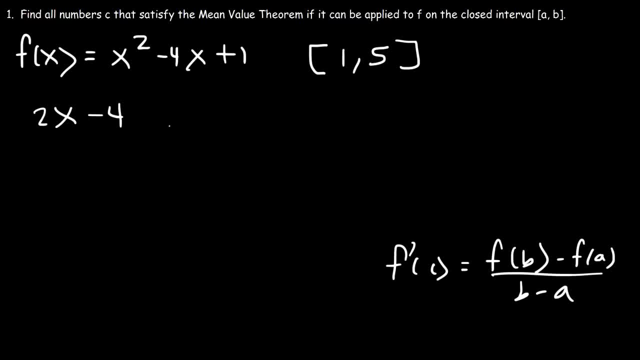 And the derivative of negative 4x is negative 4.. And for a constant it's 0. So f prime of x is going to be 2x minus 4.. And then a is 1, b is 5.. 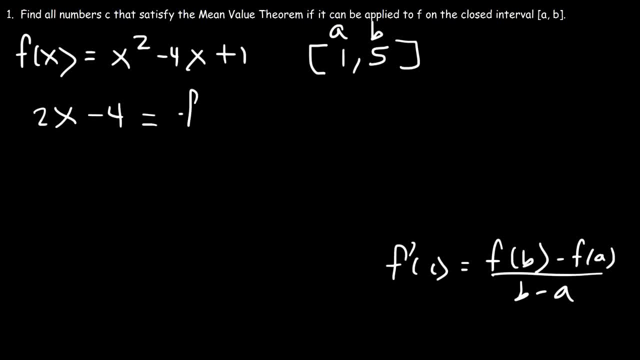 So f of b minus f of a, that's going to be f of 5 minus f of 1.. Over 5 minus 1.. Now let's evaluate f of 5 separately. So that's going to be 5 squared minus 4 times 5 plus 1.. 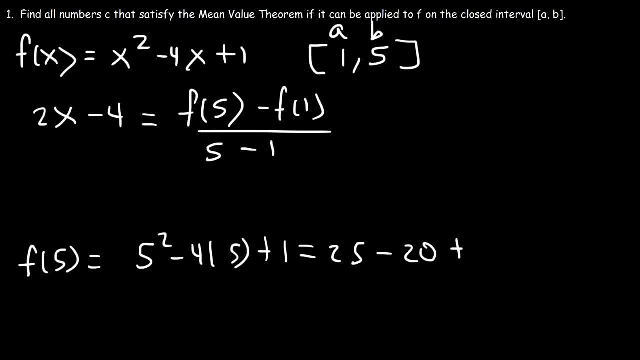 5 squared is 25.. 4 times 5 is 20.. 25 minus 20 is 5 plus 1, that's 6.. And then f of 1, that's going to be 1 squared minus 4 plus 1.. 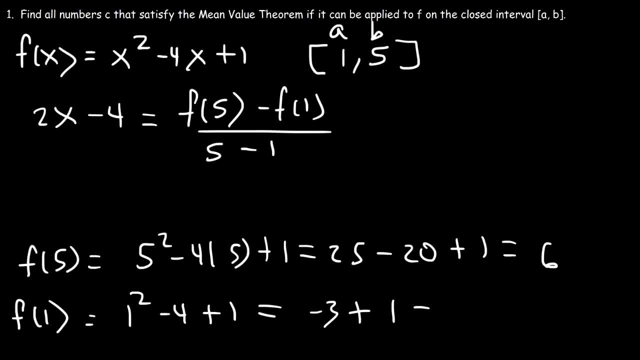 So 1 minus 4 is negative 3.. Negative 3 plus 1 is negative 2.. So we have: 2x minus 4 is equal to f of 5,, which is 6,, minus f of 1,, which is negative 2,. 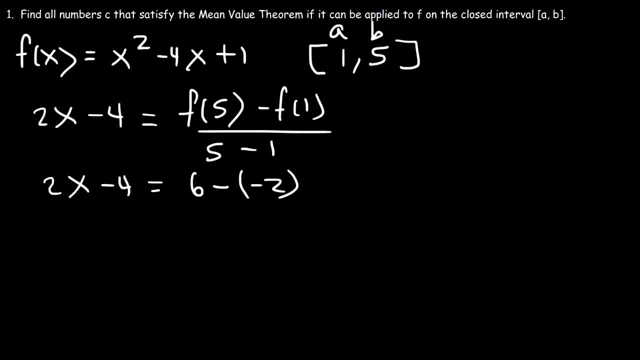 divided by 5 minus 1,, which is 4.. So 6 minus negative 2,, that's 6 plus 2.. So that's 8.. 8 divided by 4 is 2.. So let's add 4 to both sides. 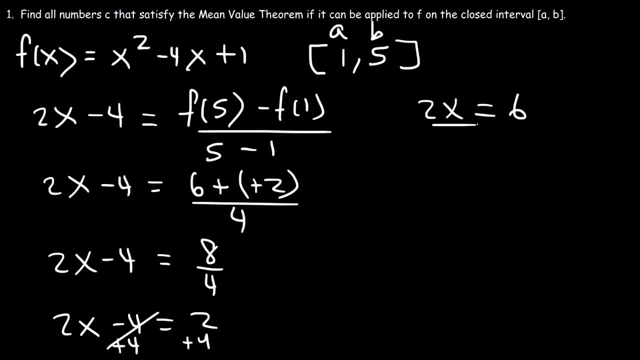 2 plus 4 is 6.. And then, if we divide both sides by 2,, we can see that x is equal to 3.. And 3 is between 1 and 5. So therefore, we can say that c is equal to 3.. 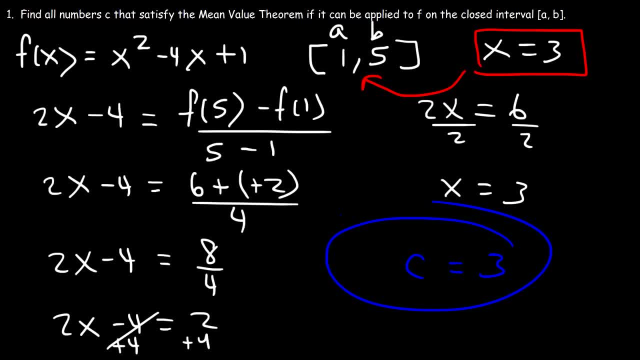 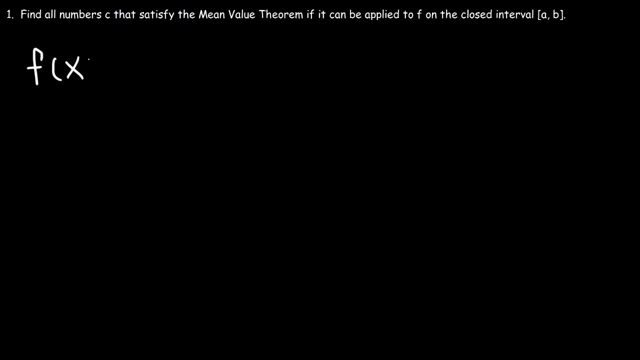 So this is the value of c that satisfies the mean value theorem over the interval 1 to 5 for this function. Now here's another example that we can work on. So let's say that f of x is x raised to the 2 thirds over the interval 0 to 1.. 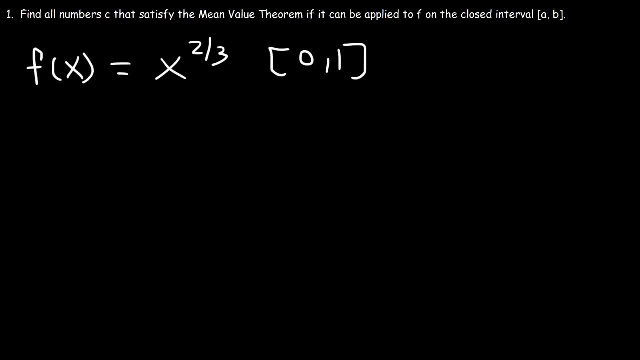 Can we apply the mean value theorem to this particular function? Well, let's find out. So let's start with a graph. x to the 2 thirds has this general shape, So we have a cusp at 0.. So what that means is that it's not differentiable at. x equals 0.. 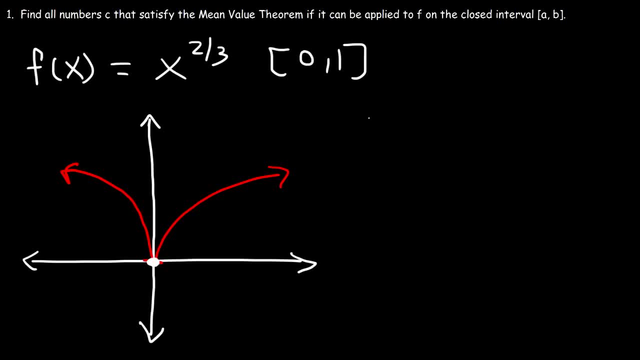 So can we apply it? Well, to apply the mean value theorem it has to be continuous on the closed interval a to b. So a is 0 and b is 1.. Is it continuous from a and b? Yes, it is. 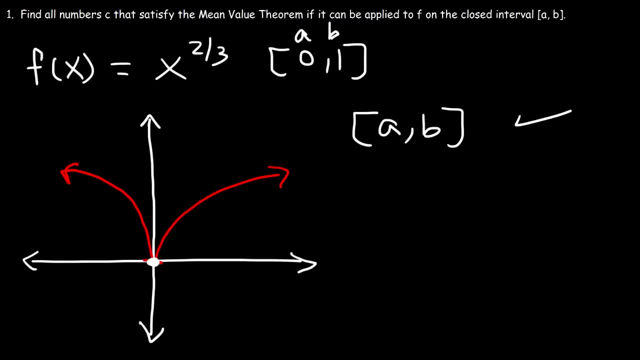 There's no jumps, no holes, no infinite discontinuities, no vertical asymptotes. Is it differentiable on the interval a, b, That is, is it differentiable between 0 and 1? Yes or no? Think about that one. 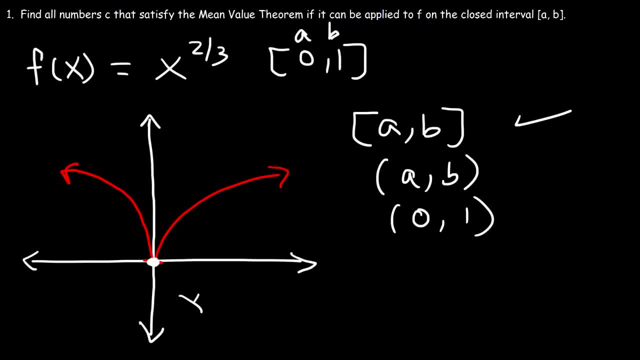 So we said that it's not differentiable at x equals 0.. Because at x equals 0, we have a cusp. Now, is 0 included in this interval? No, it's not. 0 is included in the closed interval, but not on the open interval. 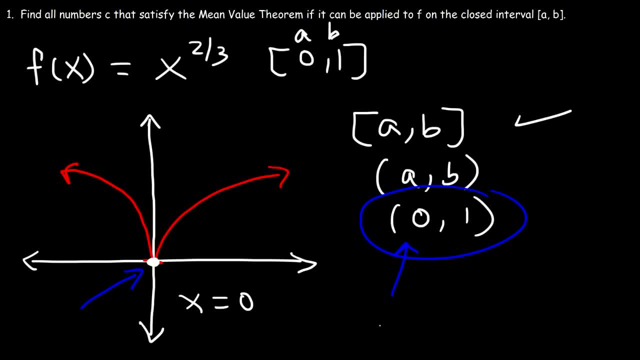 This interval tells us that x is greater than 0, but less than 1, but doesn't include 0. So therefore we can apply the mean value theorem, Because 0 is not included. So between 0 and 1, it is differentiable. 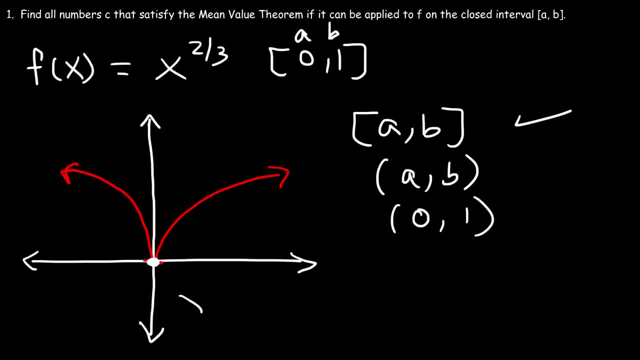 It's not differentiable at exactly when x is 0.. Now let's find the value of c that satisfies the mean value theorem for this problem. So let's start with this formula: f prime of c is equal to f of b minus f of a, divided by b minus a. 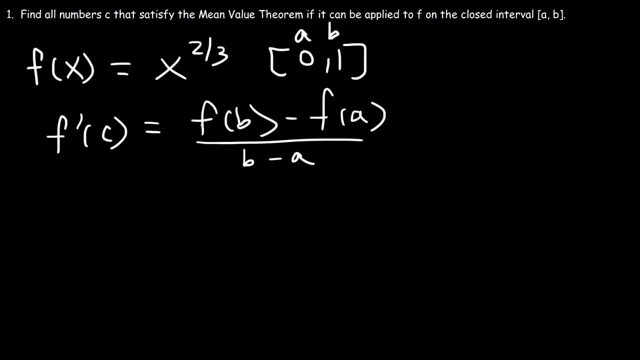 So on the left side, let's find the first derivative, Let's use the power rule. So it's going to be 2 thirds x and then 2 thirds minus 1. That's 2 over 3 minus 3 over 3, which is negative: 1 over 3.. 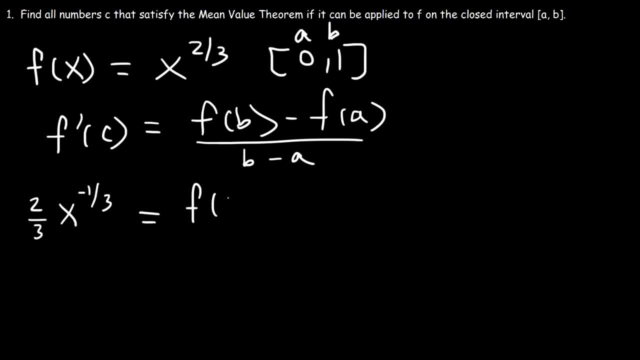 So that's the first derivative. On the right, we have f of 1 minus f of 0, over 1 minus 0. Now let's rewrite this. We can rewrite it as 2 divided by 3, x to the positive 1. third, 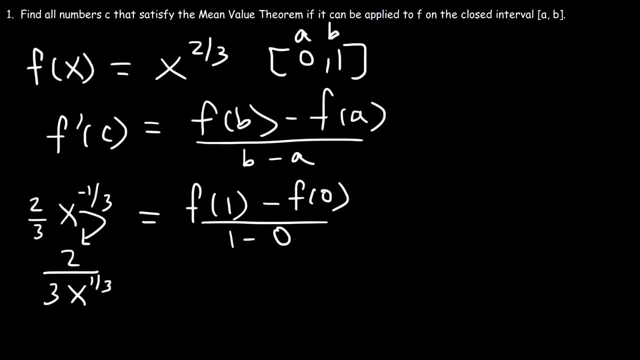 By moving x to the bottom, we could change the negative exponent into a positive one. Now, f of 1, that's going to be 1 raised to 2 thirds. 1 raised to anything is 1.. f of 0 is 0. raised to anything is 0.. 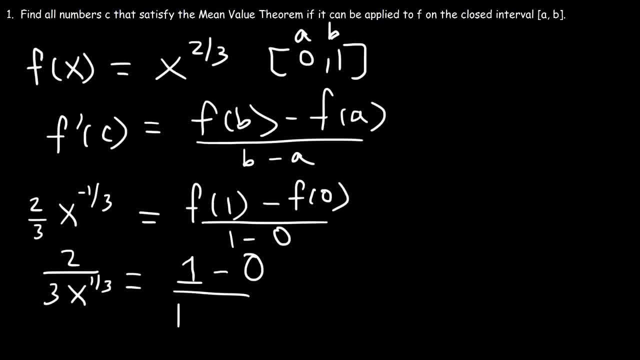 And that's over 1 minus 0,, which is just 1.. So on the left we have 2 over 3, x to the 1 third. On the right, we just have 1 over 1,, which is 1.. 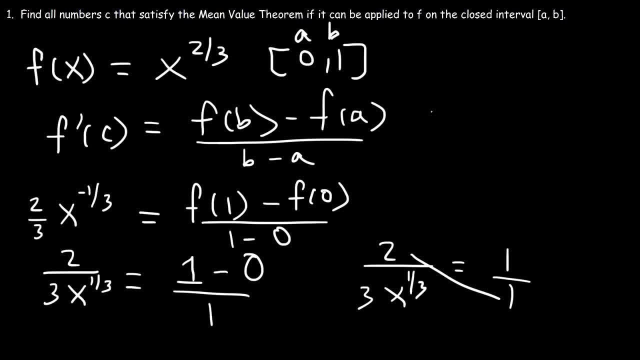 But I'm going to cross multiply. So 2 times 1 is 2.. And then on the other side we'll have 3 x to the 1 third. So now let's divide both sides by 3.. 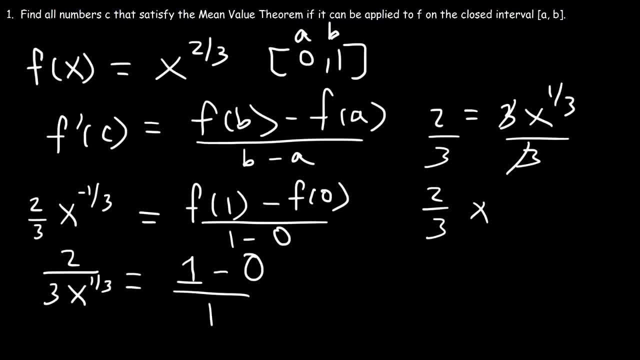 So 2 thirds is equal to: I wrote x too soon. x to the 1 third is the same as the cube root of x. Now to get rid of the cube root symbol we need to cube both sides. 2 to the third power is 8.. 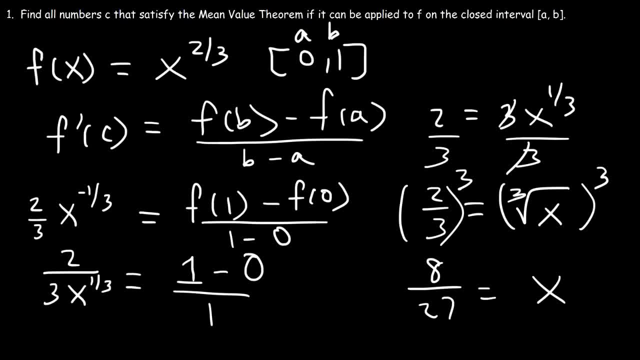 3 to the third power, or 3 times 3 times 3, that's 27.. So x is 8 divided by 27.. And to get that as a decimal, That's approximately 0.296.. 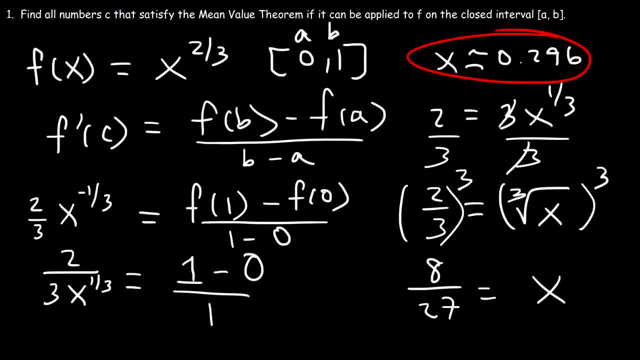 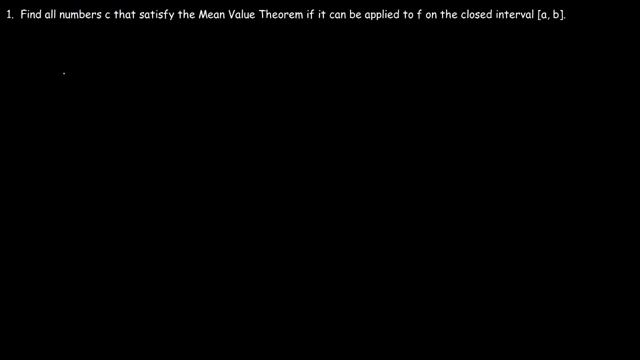 Which is between 0 and 1.. And so that's the value of c that satisfies the mean value theorem for this problem. Now let's work on this problem. An absolute value expression, Let's say if we have the absolute value of 4x minus 5 over the interval 0 to 2.. 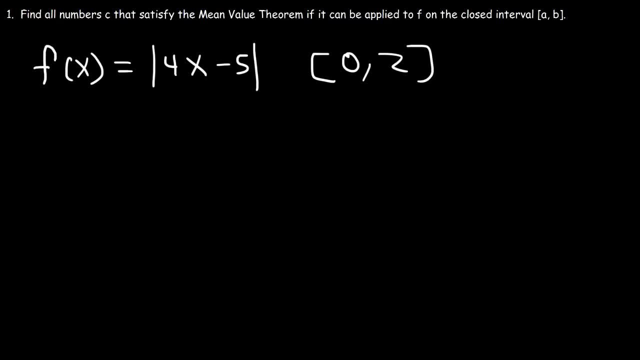 Can we apply the mean value theorem to this particular function? Well, let's start with the parent function of the absolute value of x. So it has a slope of 1, and it looks like this. So notice that it's not differentiable at 0.. 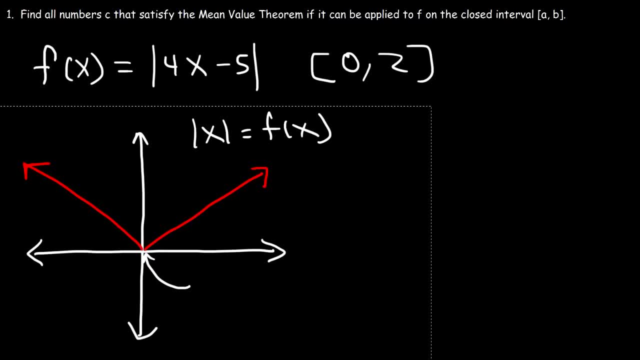 So keep that in mind. Now, how can we graph this particular function? How can we identify the vertex? To identify the vertex set the inside part equal to 0.. And so if we add 5 to both sides and then divide by 4,, 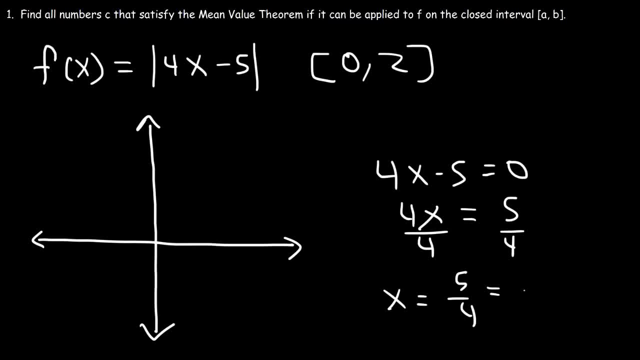 the vertex is going to be 5 over 4.. Which is, as a decimal, 1.25.. So let's say that's 1 and this is 2.. So 1.25 will be in that region. 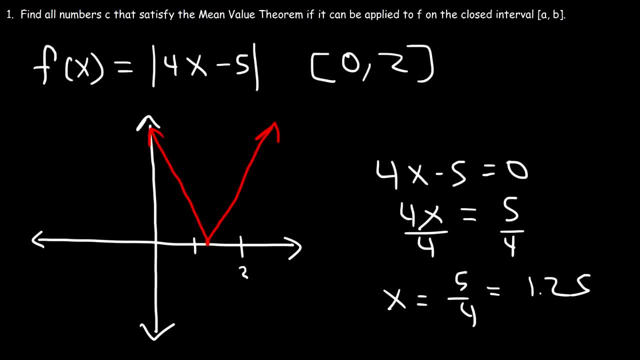 And the slope is 4.. So that's just a rough sketch for this particular graph. So is the function continuous on the closed interval a, b? Yes, it is. There's no holes, no vertical asymptotes, no type of discontinuities. 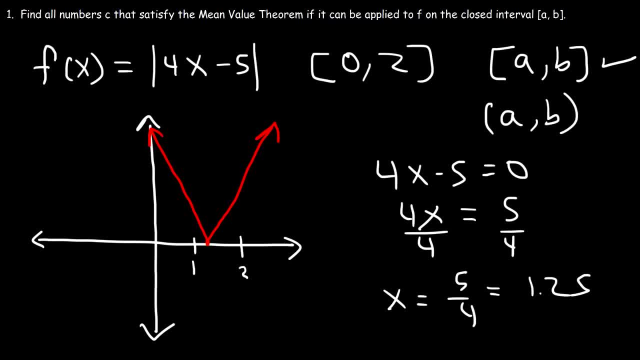 Is it differentiable on the open interval a, b, That is, is it differentiable between 0 and 2? Now we have a sharp turn at x equals 1.25.. So it's not differentiable there. And this point. 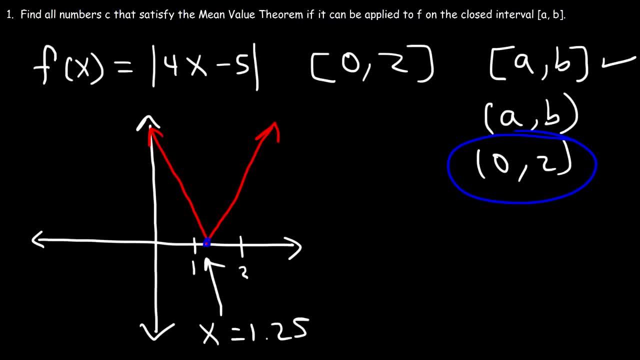 Lies inside this interval, So therefore it is not differentiable on the open interval a- b. As a result, because the second condition wasn't met, we cannot apply the mean value theorem to this problem, And so there's nothing we can do here. 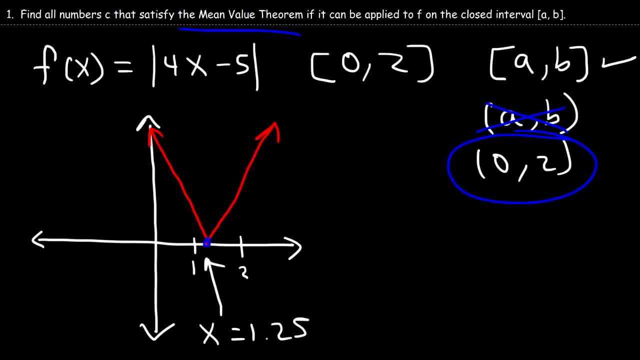 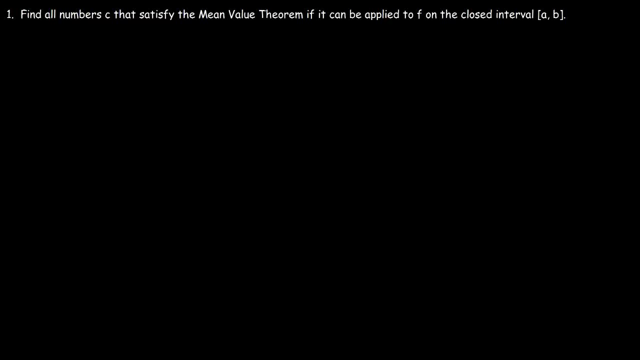 All we can say is that it's not differentiable at. x equals 5 over 4, or 1.25.. And so the mean value theorem cannot be applied. Let's work on one more problem. So let's say that f of x is equal to the square root of x minus 4 over the interval 4 to 8.. 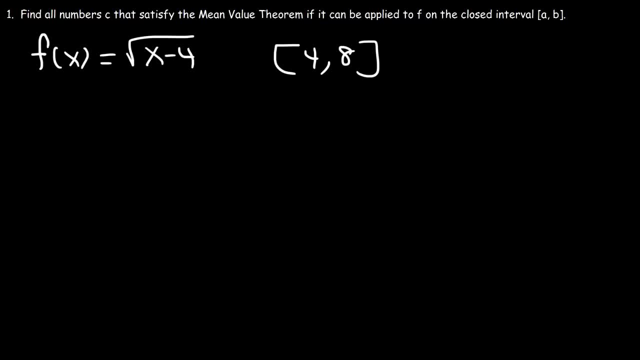 Can we apply the mean value theorem in this example? Well, let's start by drawing the graph. So let's start with the parent function. The square root of x looks like this, And so the square root of x minus 4 is going to be shifted 4 units to the right. 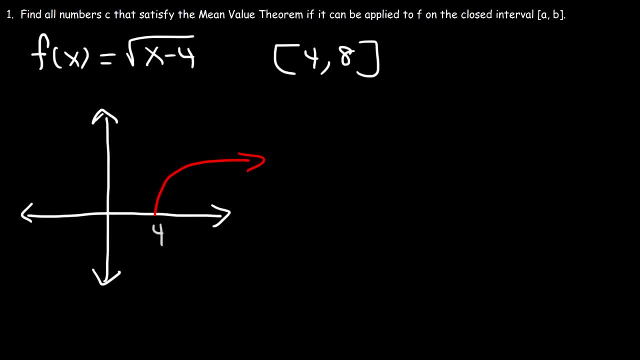 So we have a graph that looks like that. So, from 4 to 8, is the function continuous on the closed interval a to b? And the answer is yes. Is it differentiable on the open interval a- b, Since there are no sharp turns, the answer is yes. 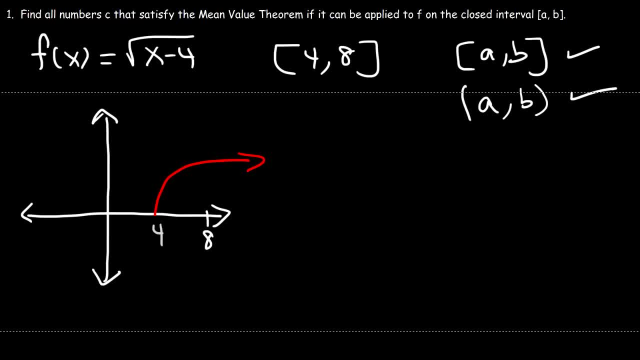 So therefore we can apply mean value theorem to this particular problem. So let's start with this equation: f prime of c is equal to f of b minus f of a divided by b minus a. So in this example we can see that a is 4 and b is 8.. 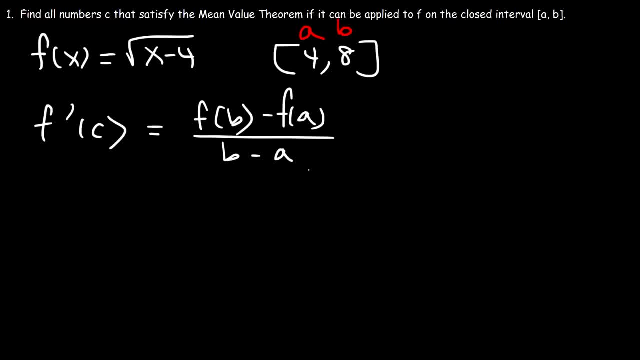 So first let's find the first derivative. We can rewrite it as x minus 4 raised to the 1 half, So it's going to be 1 half x minus 4.. And then 1 half minus 1 is negative 1 half. 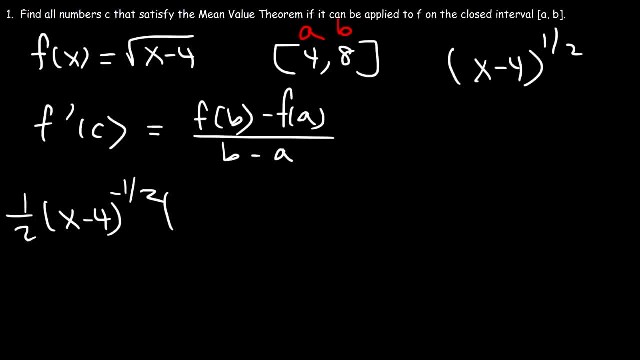 And then the derivative of the inside function x minus 4 is 1.. And that's equal to f of b minus f of a over b minus a. So now let's rewrite this expression. We're going to move this to the bottom to make the negative exponent positive. 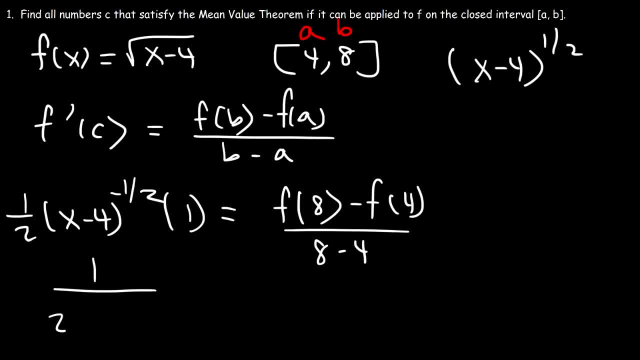 And so it's going to be 1 divided by 2 times x minus 4 raised to the 1 half, And that's going to equal f of 8, which is the square root of 8 minus 4.. And then f of 4, which is the square root of 4 minus 4.. 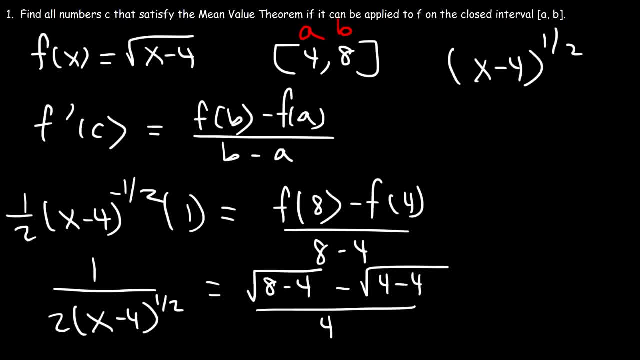 And then 8 minus 4 is 4.. So on the left we can rewrite that as the square root of x minus 4.. And then 8 minus 4 is 4.. And the square root of 4 is 2.. 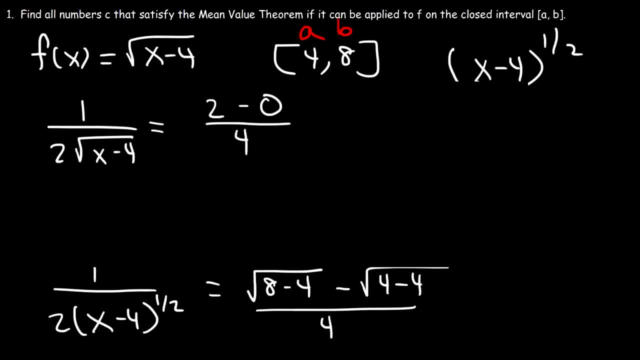 4 minus 4 is 0.. And so this is what we now have, And if we cross, multiply now 1 times 4 is 4.. And then 2 times 2 is 4. And then we could divide both sides by 4..